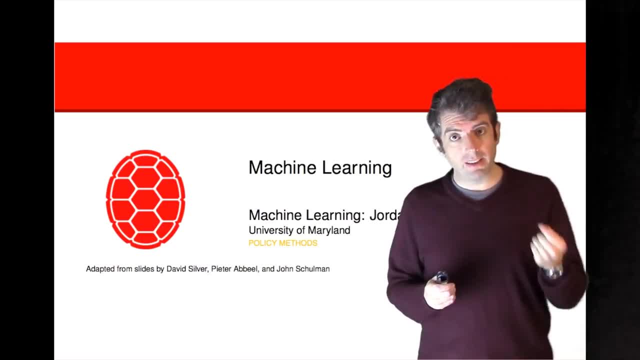 We're going to continue our discussion of reinforcement learning, but today we're going to focus on some of the more recent advances from deep learning. And deep learning has reinvigorated the subfield of reinforcement learning, And so, whereas before it used to, 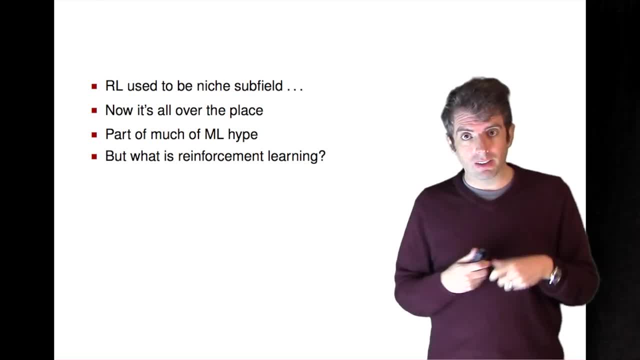 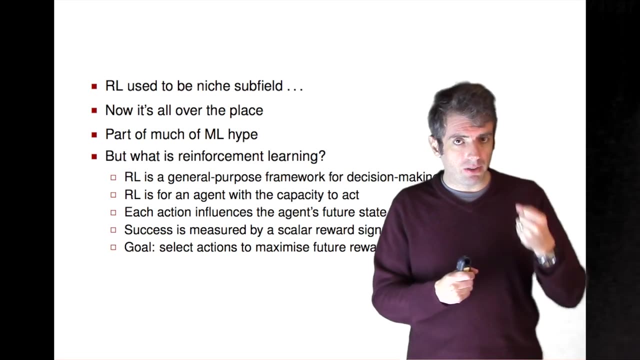 be a relatively niche part of the machine learning community. things like AlphaGo and the success of playing Atari have really reinvigorated reinforcement learning as a very hot area inside machine learning. And just to refresh your memory, reinforcement learning is where you have an agent that needs to take actions in some state space and as it takes those. 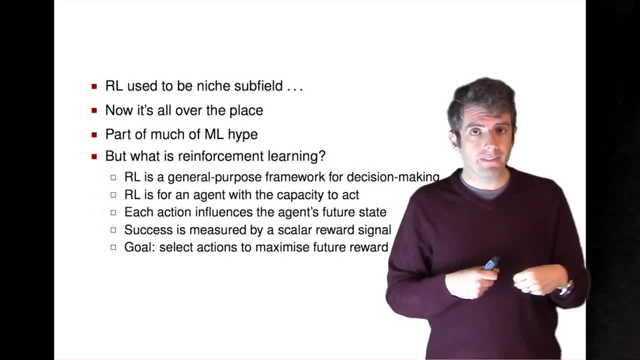 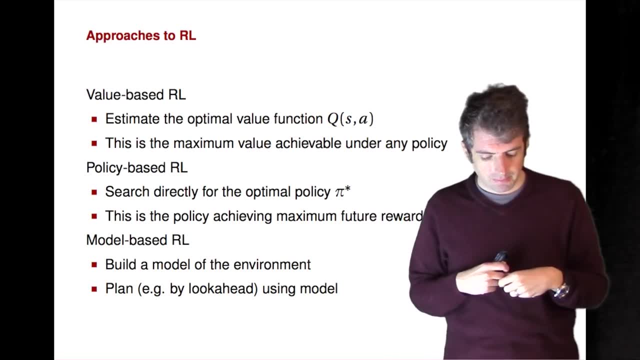 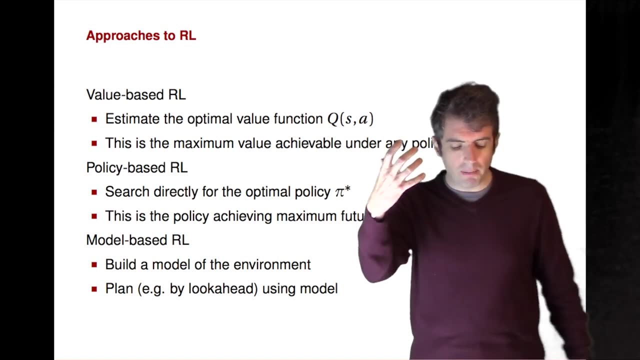 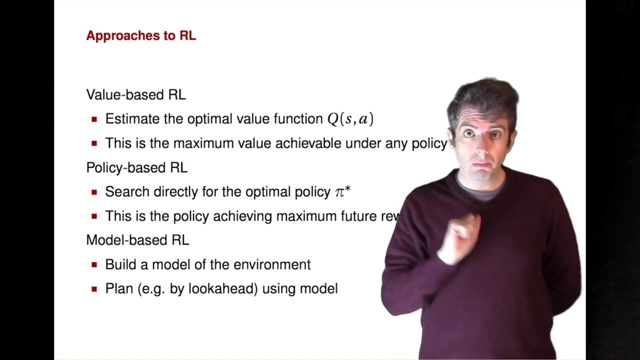 actions, it gets a reward And the learning problem is difficult because you have a problem of delayed rewards that the agent needs to internalize. Three: two: So we began talking about value-based reinforcement learning, where we tried to explicitly learn Q or V functions to tell us what to do in particular states. Another: 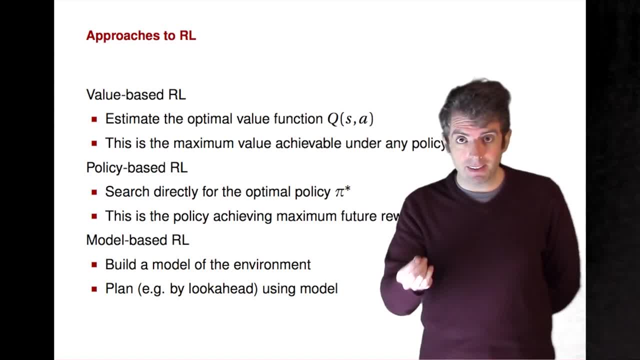 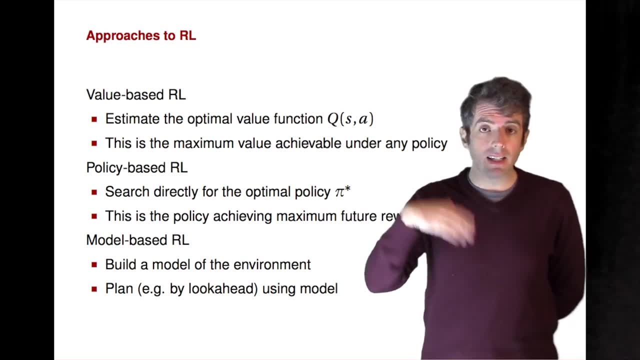 way of solving reinforcement learning problems is using policy-based methods, where you try to explicitly learn a policy, either through searching your space or by, say, imitating an expert. The final class of reinforcement learning that we're not going to talk about at all is model-based reinforcement learning. that requires a lot more world knowledge and 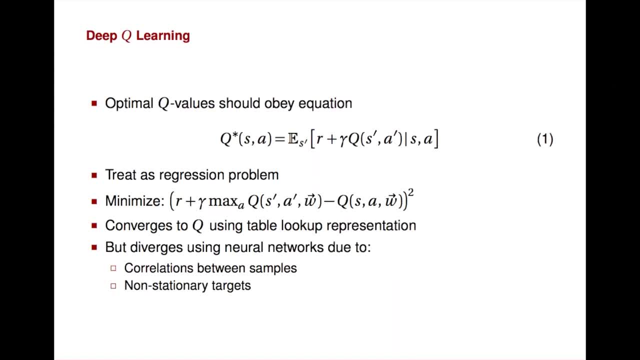 is more task-specific. We talked about Q and V functions. and we talked about Q and V functions. We talked about Q-learning before, but you can also apply deep learning methods to do a better job of Q-learning. Recall that Q-learning is learning a lookup table If you're in state. 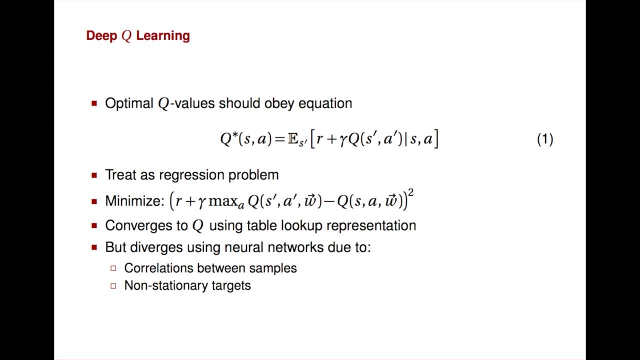 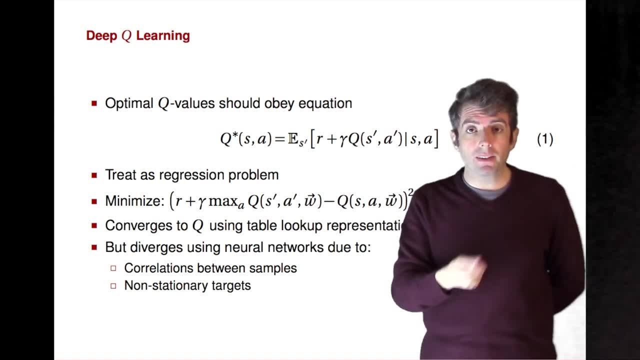 S and take action A. what is your expected reward? moving forward- And before, we treated this as a lookup table problem- but we can treat this as a regression problem as well- You take your representation of the state vector in some form and you use that to predict. 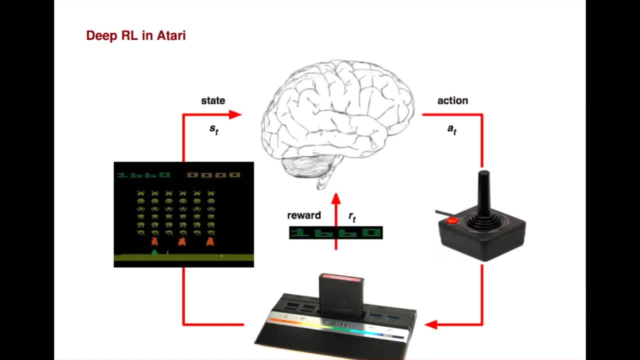 what the Q value will be. This was used quite successfully and to great publicity in getting deep learning to play Atari games. The nice thing about games, as we've talked about before, is that you have this nice score element that serves as a good proxy for the reward that. 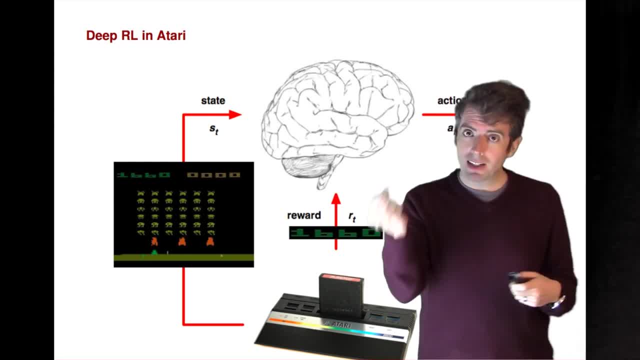 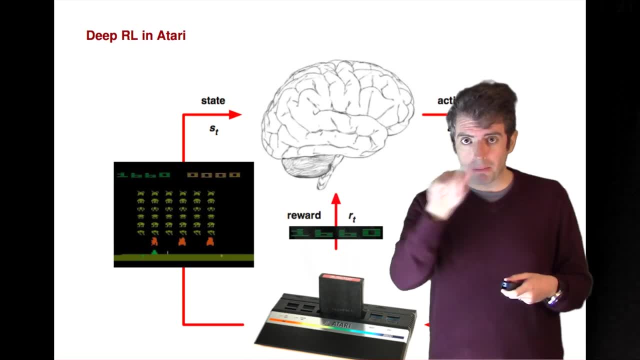 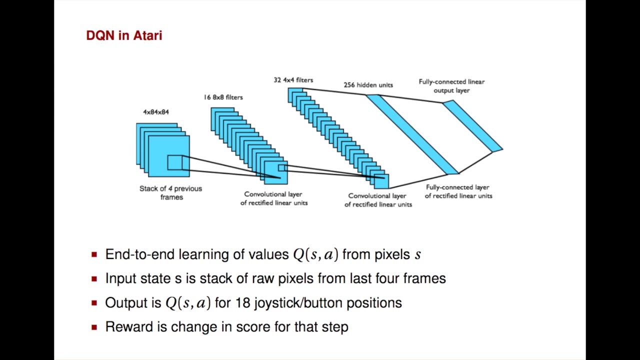 you should get in reinforcement learning. Your action space is, say, moving around an Atari controller in one of the eight directions and pressing the fire button. The state is just the image of the screen. What they did is they built a system that takes the screen. 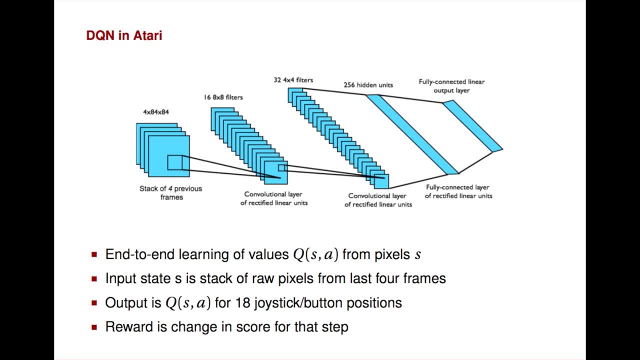 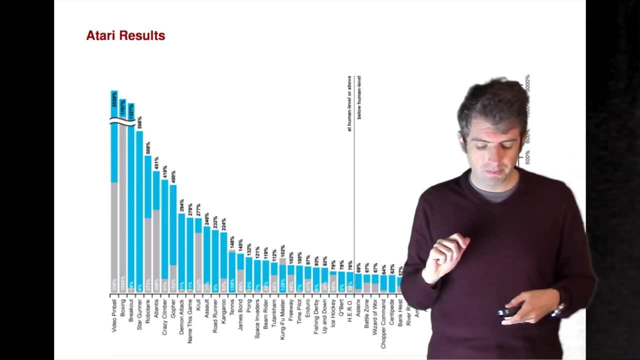 input passes in through a number of feedforward units in a deep learning model and then tries to predict what the Q value is for a state-action combination, Then the score change gives you your reward. So they were able to do very well in a number. of Atari games. They were able to fix some problems with the data. That might have been harder to do in a previous video, but you can go through a lot of different examples of this. It's going to help you with a lot of different problems For this video I'm actually going to show you. 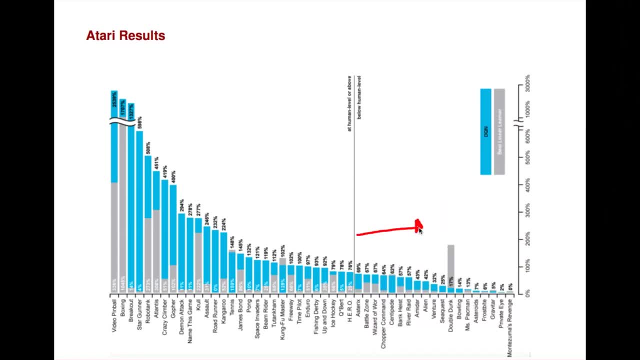 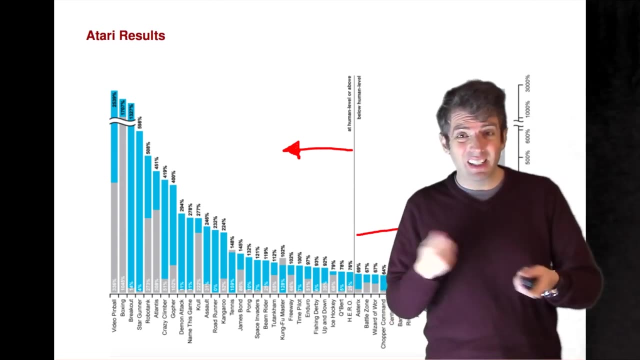 And so for a number of games they're still not up to human performance, but for many games they're able to do better than human performance, And this is really exciting, because this is not using any sort of knowledge about the rules of the game. 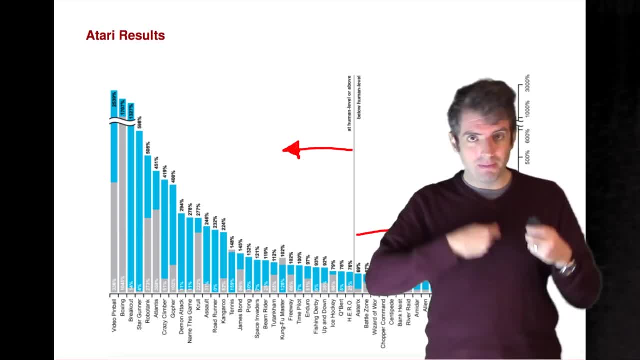 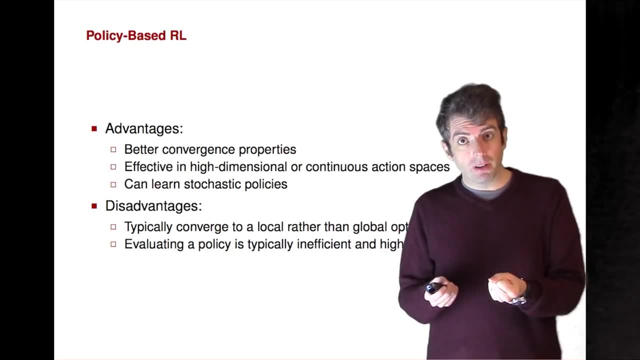 not even reading the handbook but just experimenting by moving the joystick around in random directions and seeing how the score changes. But the deep Q learning approach has some issues. It doesn't necessarily always converge to good values And one of the responses was trying to learn the policy directly using deep learning. 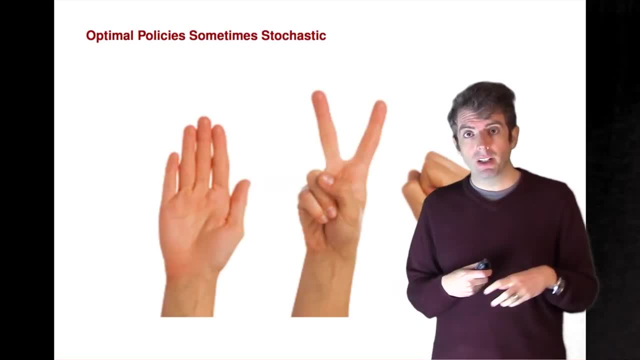 One of the advantages of using a policy-based approach is that you can learn stochastic policies. For example, if you're playing Rochambeau or Rock Paper Scissors, the best policy is to randomly select one of the actions And 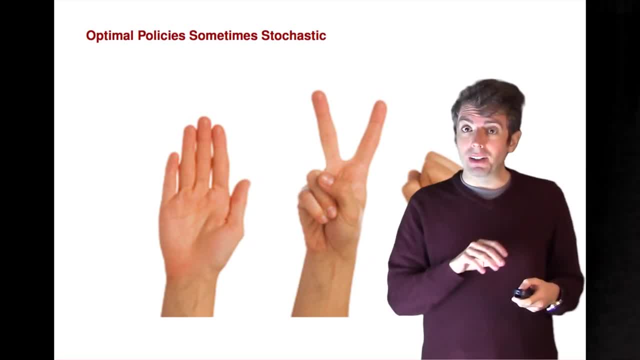 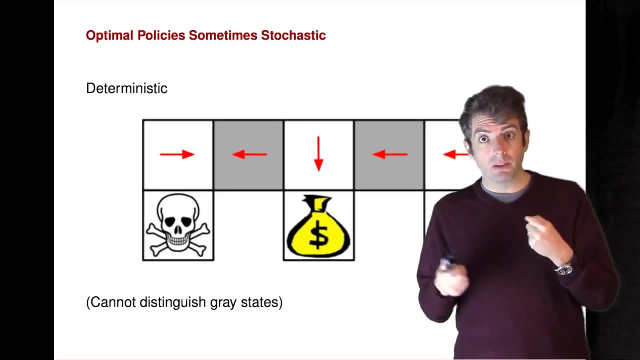 And to ignore your history. This is difficult for Q learning to do. So, for example, let's say that you're in a world that looks like this and your agent cannot distinguish the gray states, And if you did something like Q learning, you would learn in a gray state to go either left or right. 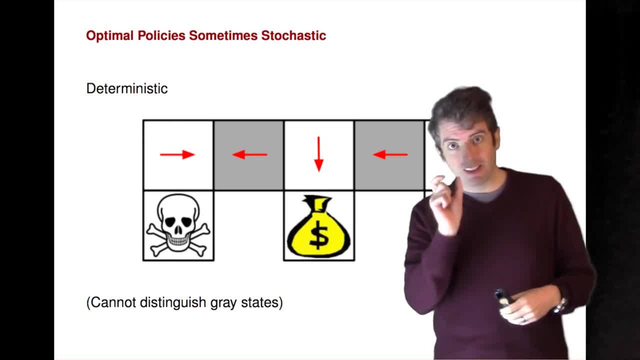 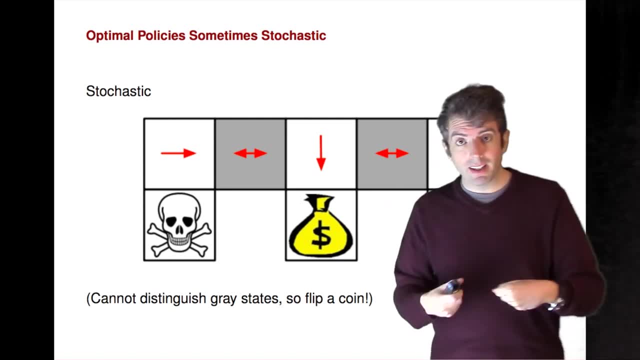 You have some argmax over the various state-action combinations, But what you want to do is to be able to learn that if you're in a gray state, you should flip a coin and then go either left or right. That is the optimal strategy. 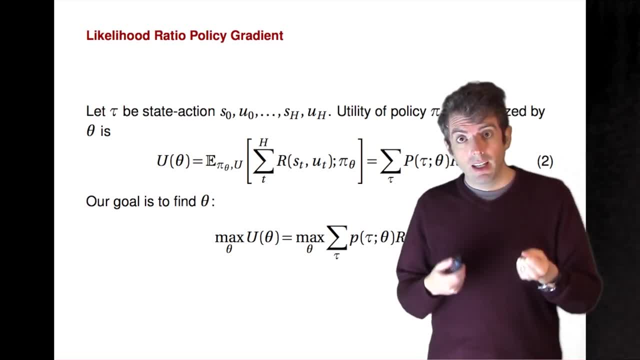 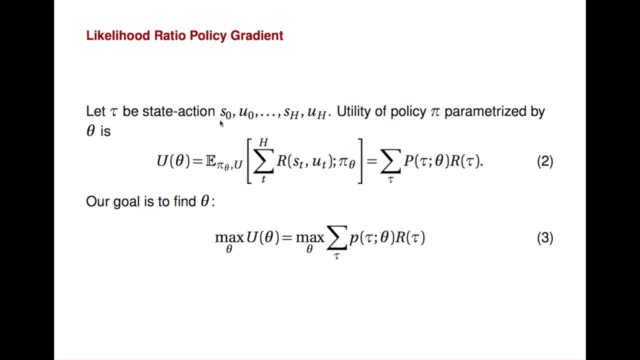 So is there a way that we can parameterize the policy-learning mechanism so that we can do things like gradient descent on the policies? So what we're going to do is we're going to create a utility function u And given some trajectory of state-action pairs. 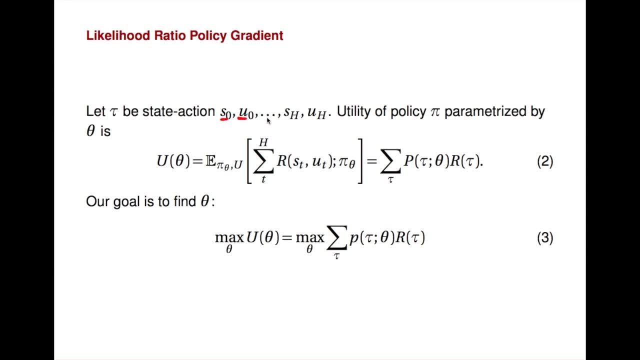 and we're going to call these. We're going to call these s and u. We want to know how good of a trajectory was that? So, for the sake of notation, we're going to call these state-action sequences tau for trajectories, And we're going to evaluate the utility by asking: given our policy. 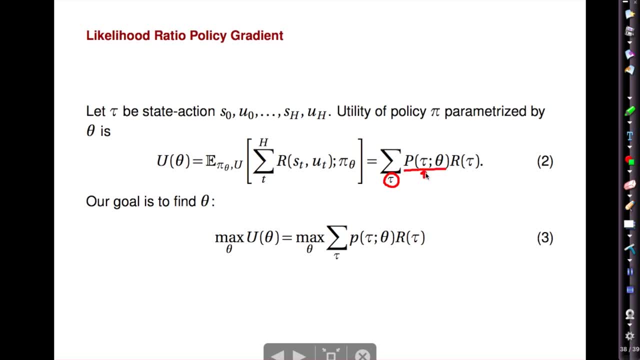 what's the probability of seeing that trajectory tau, And recall that our policy is parameterized by theta, And so this is just saying how likely are we going to be on some trajectory tau? And then, given that tau, what's the reward of that trajectory? 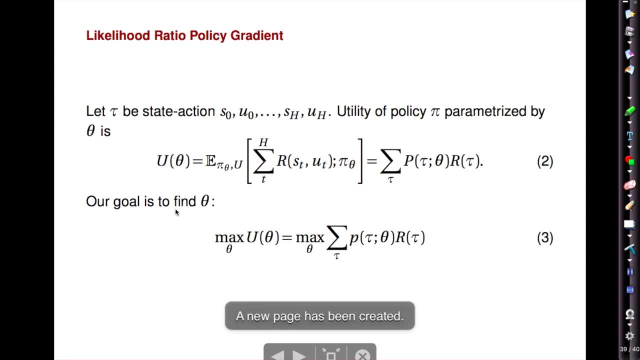 So that defines our objective function And this is going to be the utility of that policy, parameterized by theta. Okay, Given that definition, what we want to do is we want to figure out the theta that we're going to be using. 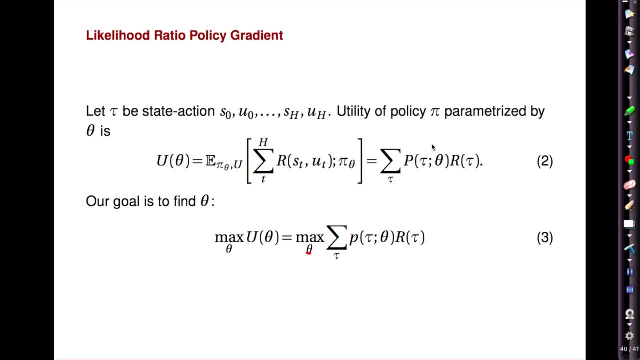 So let's try to maximize this function over theta And recall, when we're doing optimization, we're going to try to do something like gradient ascent, gradient descent, So we need to be able to take the derivative of this thing. So let's take the derivative with respect to theta. 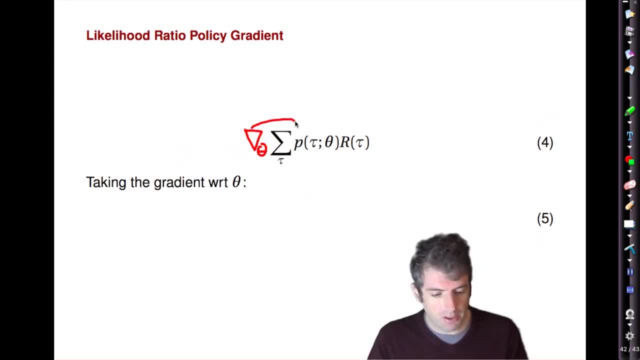 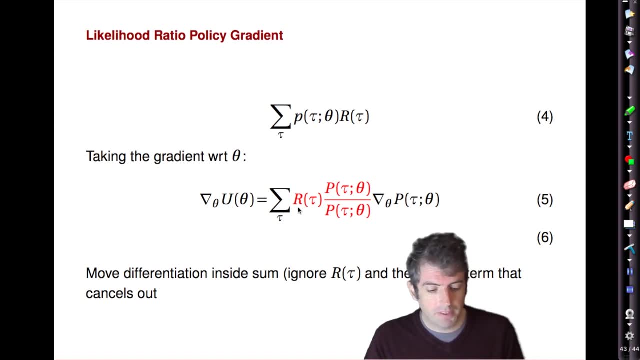 And so the first thing that we're going to do is we're going to move the differentiation so that it applies to the part that actually cares about theta. So after we've done that, the r can come to the front, And then we're going to multiply by something that is equivalent to multiplying by 1.. 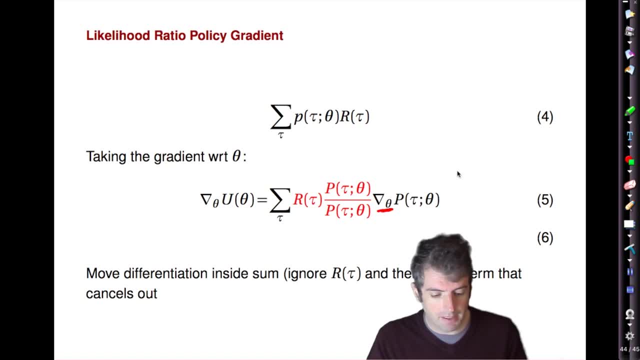 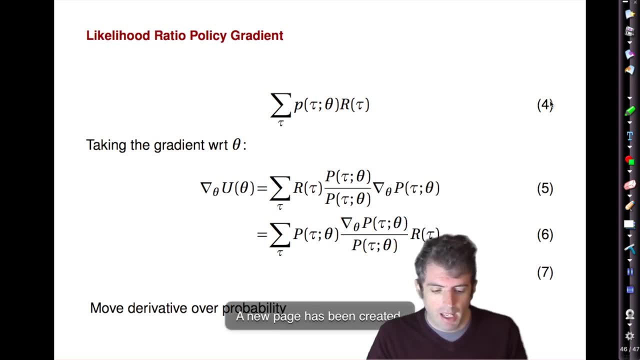 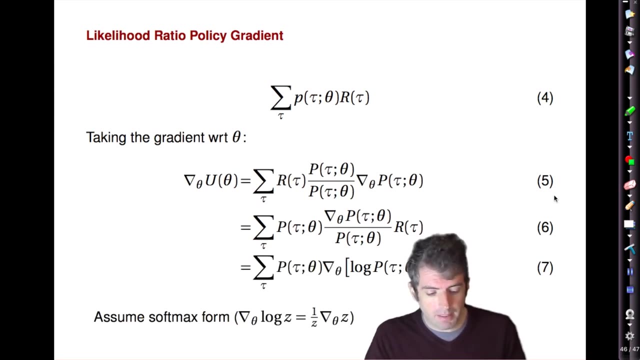 Okay, so we've moved the differentiation inside of the sum and ignored r. So this is interesting. So think for a moment: if we have a probability function that looks something like a softmax term And if our probability looks like a softmax term, we can replace 1 over z times the derivative of z with the derivative of log z. 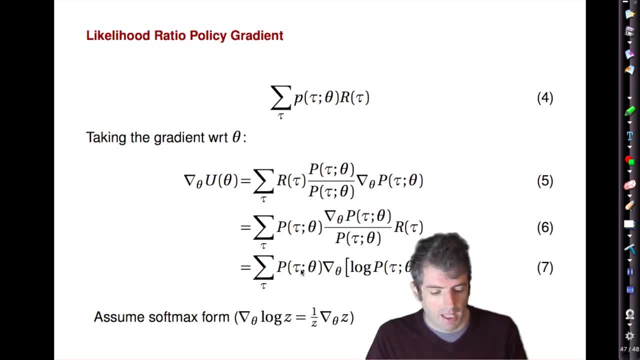 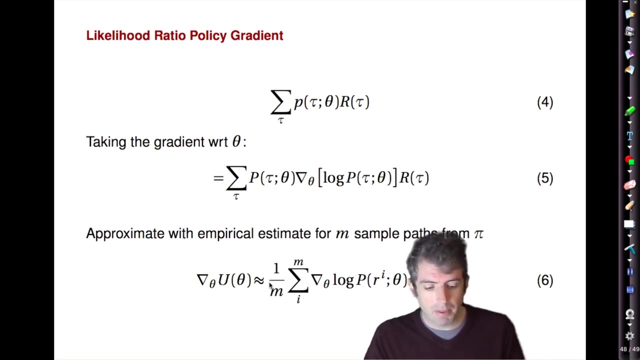 So that gives us a nice log likelihood term, And then we also have a sum over trajectories times the probability of the trajectory. So this looks a lot like an expectation And we can approximate this by taking an empirical expectation, by sampling a bunch of paths from our policy. 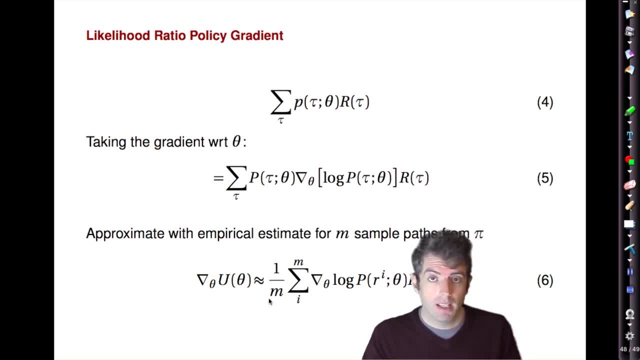 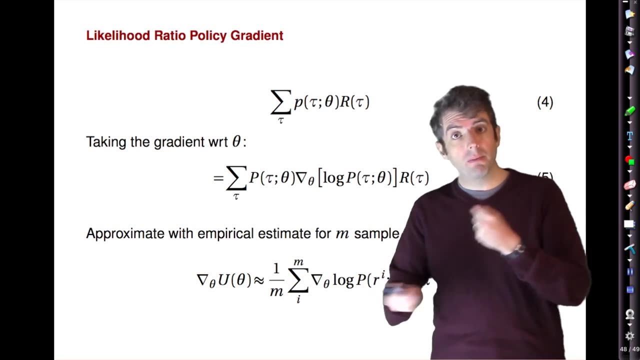 And so now we have a way of computing the derivative of the policy parameters based on a bunch of empirical samples from that policy, which is what we need to update the policy. So now that we have this, we can apply the same kinds of stochastic gradient descent. 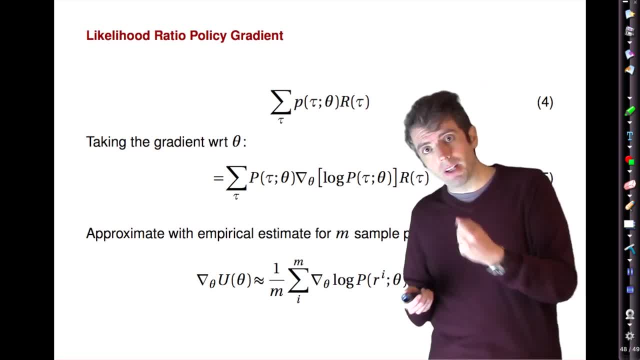 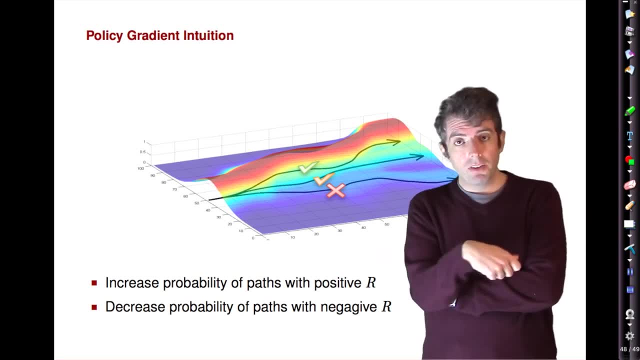 that we've applied before to our policy and learn updates that way. So now that we have this way of updating our policy, we sample a bunch of paths, and those paths will go through various parts of our state space and receive some reward. 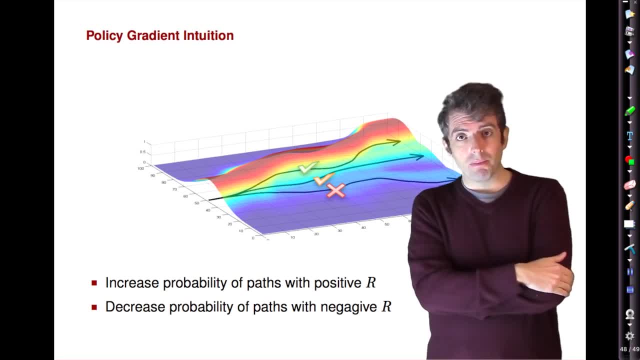 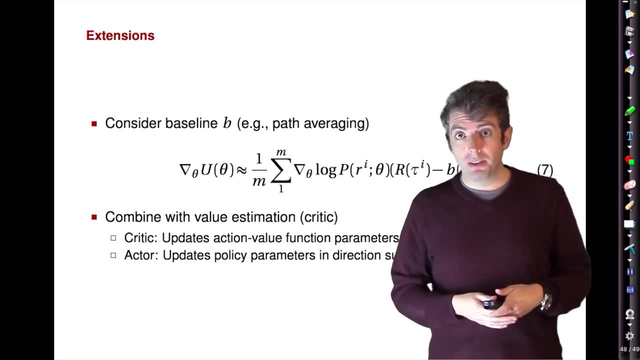 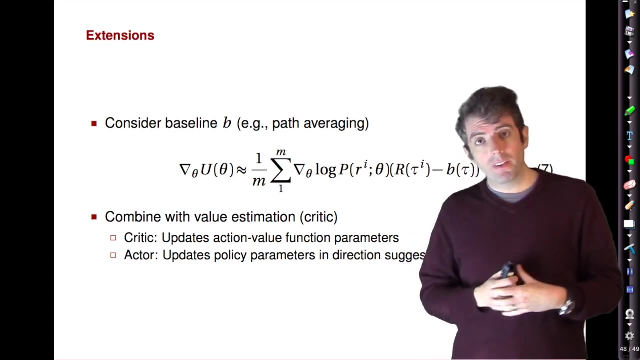 And the paths with lower rewards will have the parameters that cause them to go down those paths to become less likely. There are a lot of extensions to these policy learning techniques, and this is a very active field of research. One of the ways that you can improve this is by say: 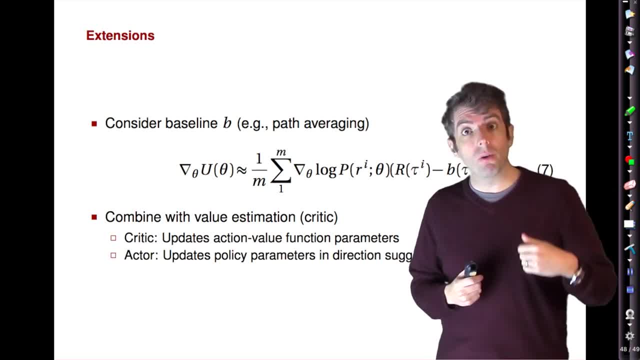 adding in a baseline policy that should work okay most of the time, And if you do this, you can make sure that your algorithm is improving over this baseline, And so you only want to reward policies that do better than some very simple baseline policy. 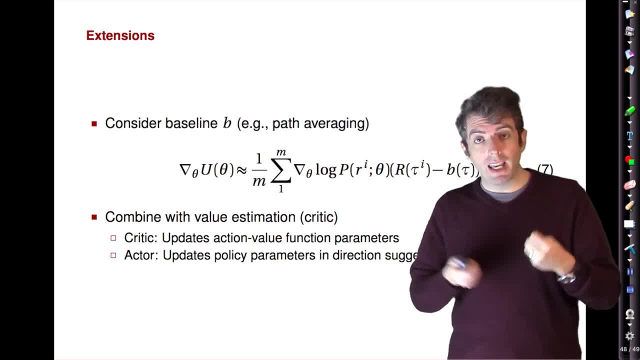 So, for example, maybe you could code up an agent by hand that does a reasonable job and you're trying to encourage your algorithm to improve over that baseline. One way of taking this to the next level is combining it with value learning, So a lot like the adversarial frameworks that we talked about before. 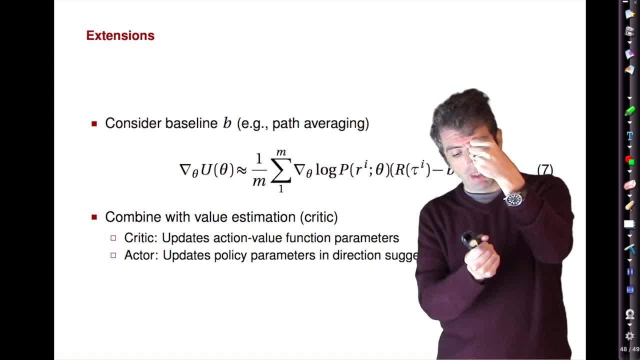 you now have an algorithm with two discrete components. The critic is trying to figure out where the reward is, The actor is trying to learn a policy, And the two of them work together to figure out where the policy is. So the critic is learning where the reward is. 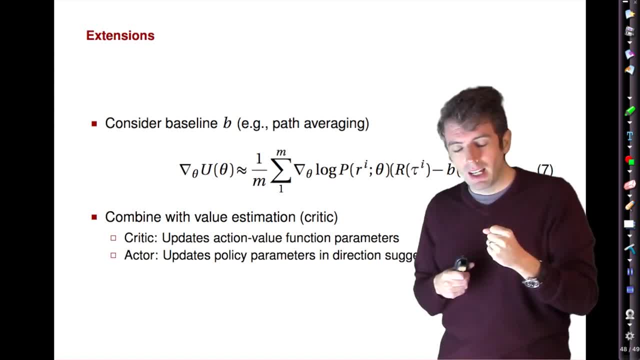 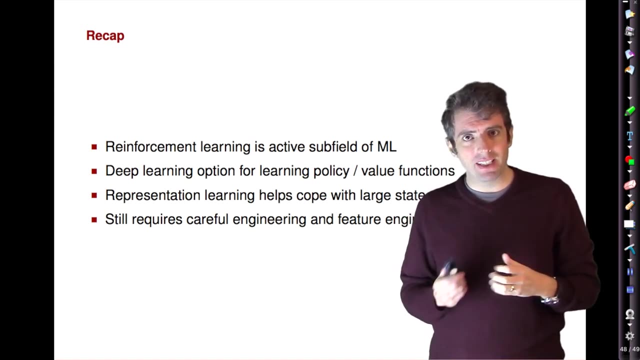 based on the policies that the actor has explored, and the actor, based on the critic's estimate of the reward, is moving the policy direction to favor high-reward areas. So, to wrap up, reinforcement learning is a very popular field of machine learning. 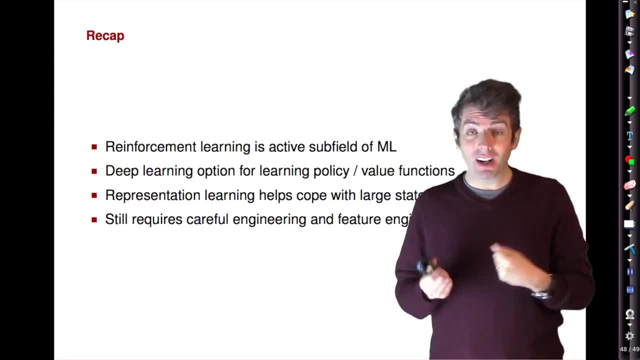 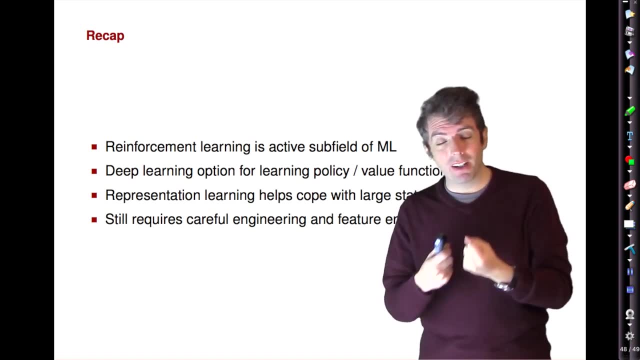 and we don't have enough time to talk about this in depth. It really deserves a course unto itself And hopefully we've talked about enough so that if this is something exciting to you, it's something that you can explore in a future course or on your own in independent research.